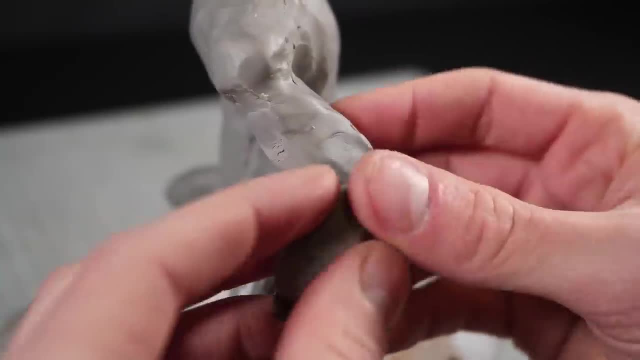 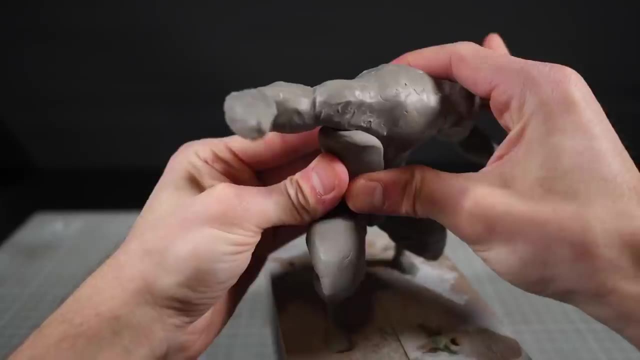 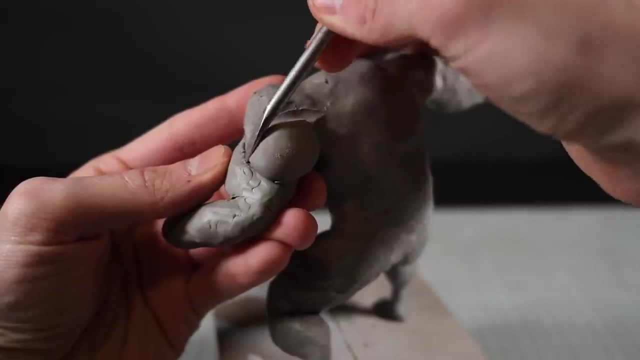 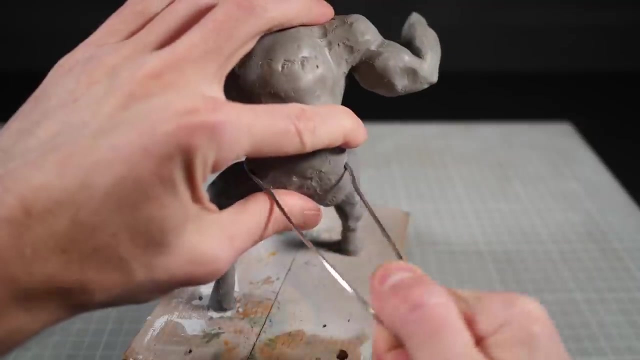 I'll start marking out where I want the muscle to lie. I want him to retain his bipedal, overly muscular upper body, so I'm going to lean into the ridiculously large muscles. Once I've got most of the muscle built up and roughly shaped, I'll wrap the torso with some 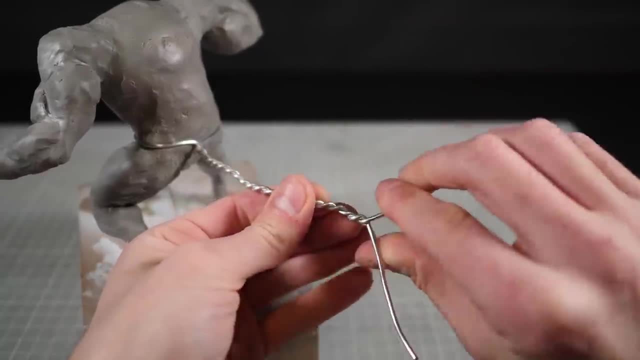 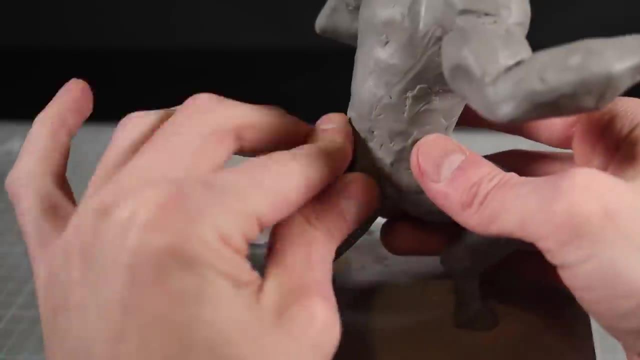 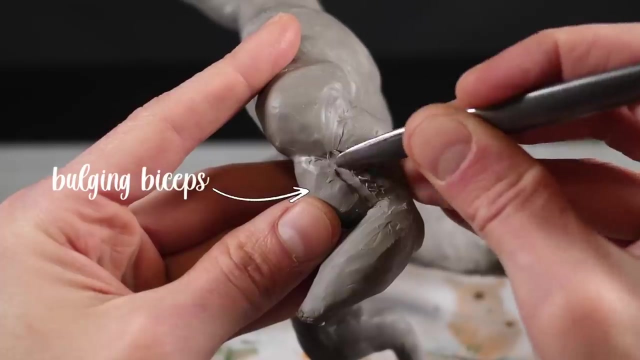 wire and then yank it tight. This will give me a nice, secure bit of wire to build my tail on top of, And I'm ready to really make this Bowser obscenely buff. We're talking bulging biceps, terrifying triceps, bolder shoulders, tree trunks for legs, and you get the point. 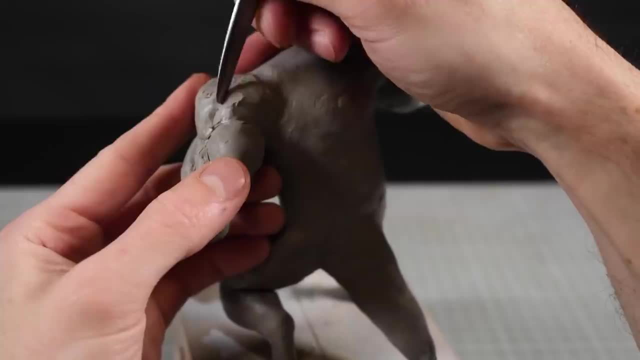 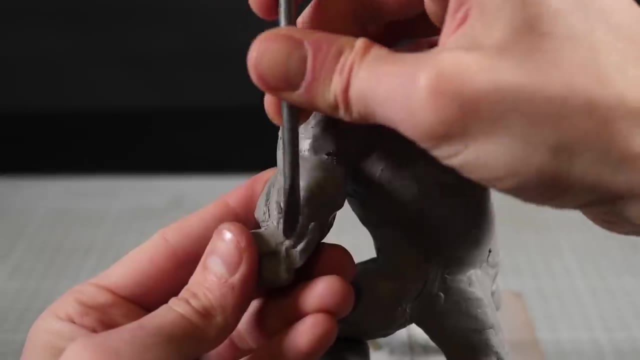 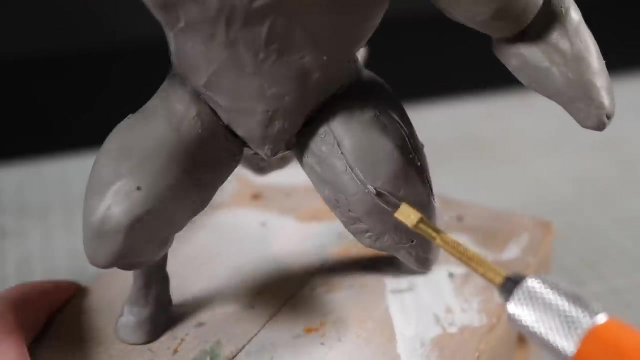 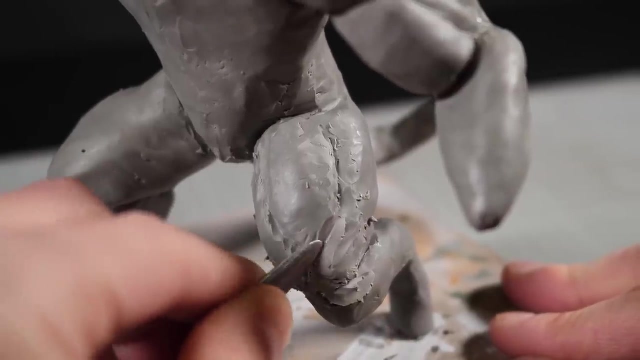 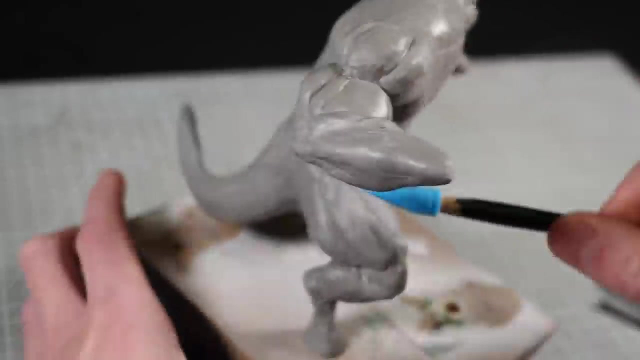 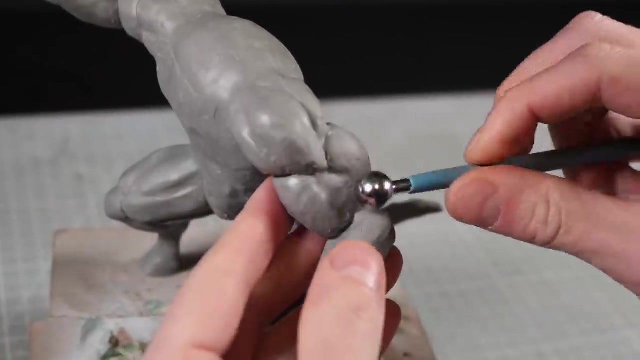 Basically, he's going to be jacked, And then, once I've cut out all the individual muscles, I'll gently blend them all together, which should leave me with a more realistic looking, albeit still shockingly muscular, King Koopa. Finally, before I get to the surface detail, I'll make his feet by squishing some small 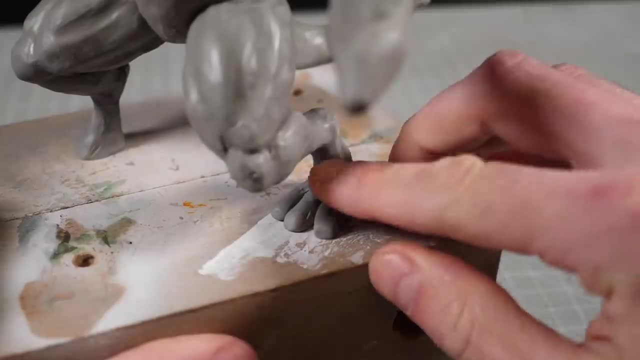 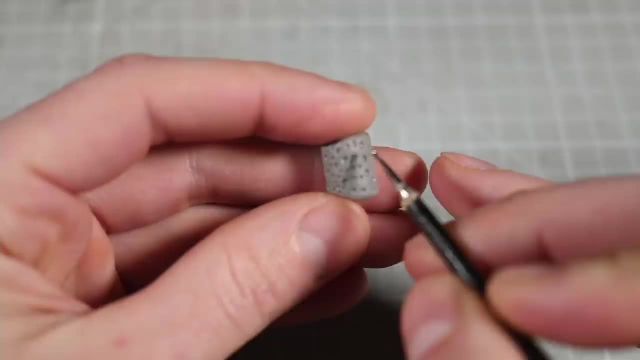 sausages onto his horse hooves and then adding a tiny bit of detail on top of those. Now, as far as surface detail is concerned, there's a few options, but I tend to lean towards the easiest, because I'm kinda lazy. I want to give Bowser's skin a scaly texture, but the idea of adding all those scales makes 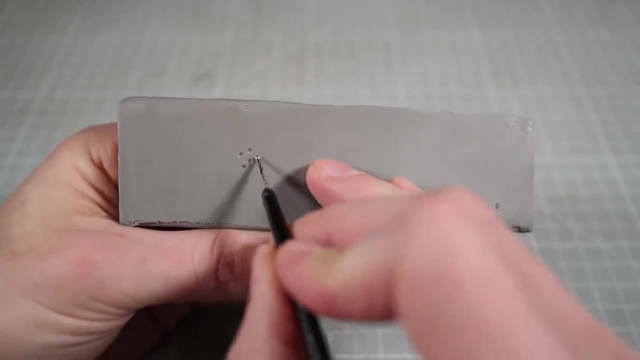 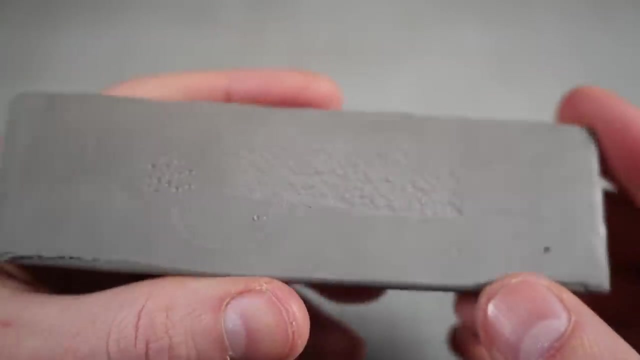 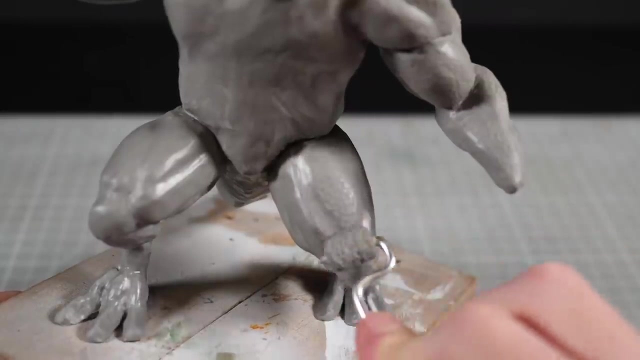 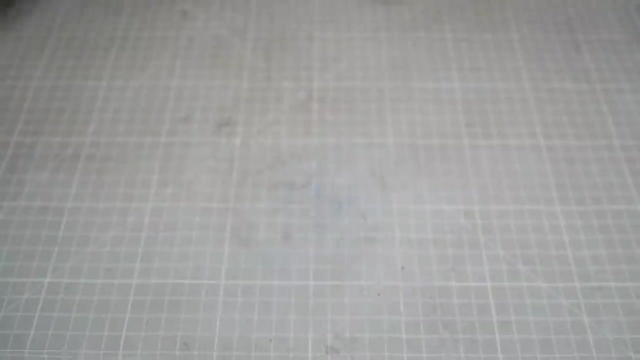 my balls itch, so instead I'm going to make a tiny, adorable texture roller, Poking tiny indents into the clay, then baking it. it should allow me to apply textures to a smooth surface And, as far as easy and lazy is concerned, you can't really argue with those results. 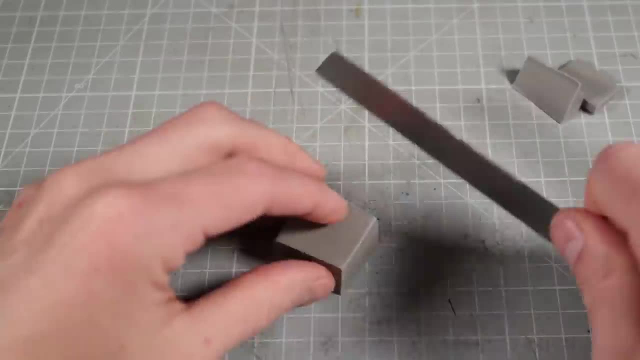 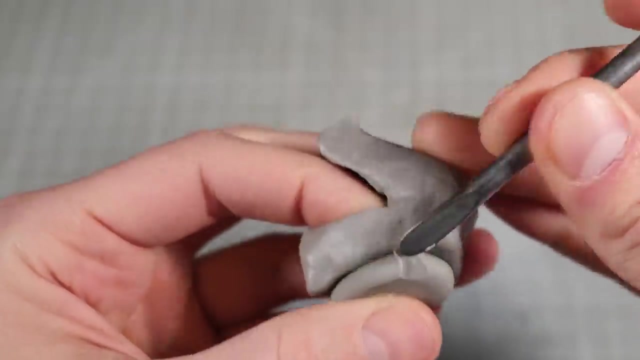 With the body mostly finished, though it's time to make his head. I'll start with a solid block and then work my way towards a somewhat recognizable face. I'm trying to keep a balance between Bowser's immediately recognizable facial features, while still allowing room for a more realistic style. 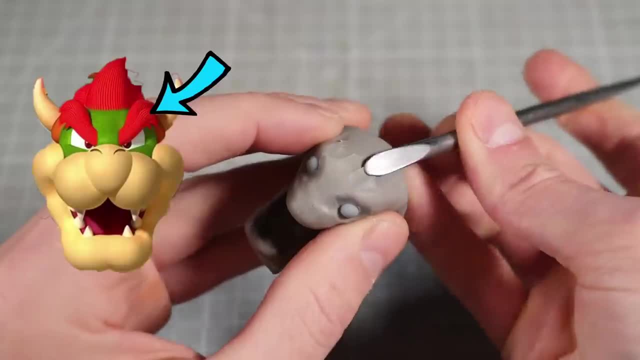 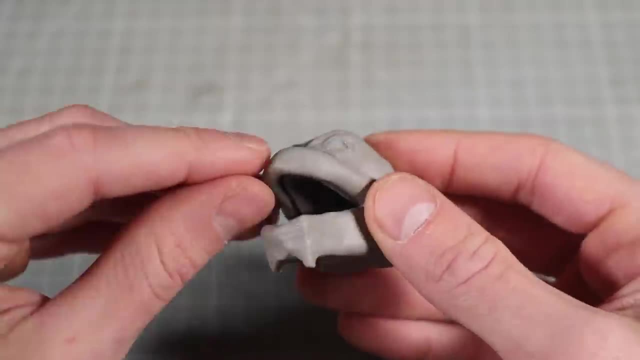 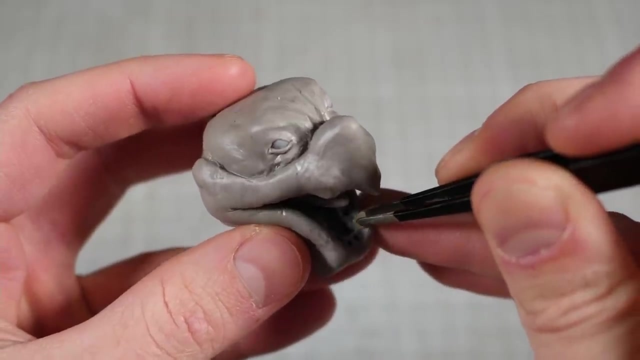 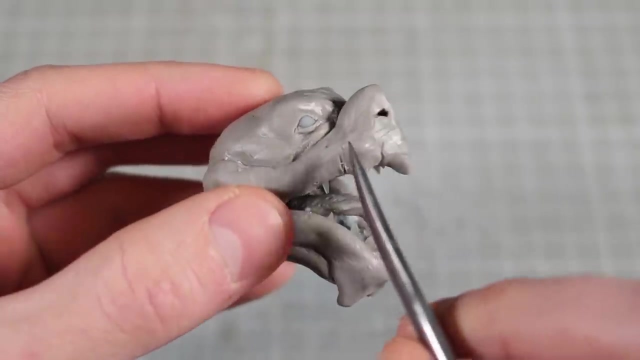 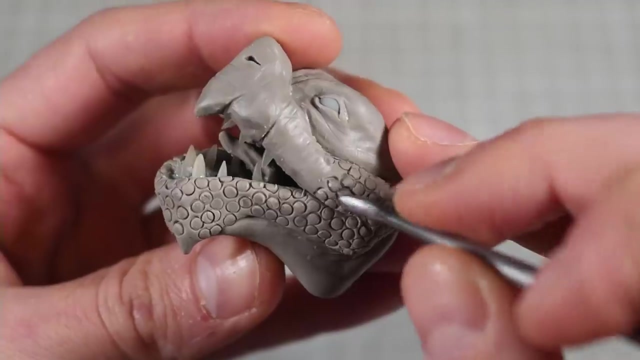 Fortunately, Bowser has some pretty big identifiers like his fiery red eyebrows and his bulbous nose slash upper lip area. I think that as long as I can keep those in place, I can probably get away with a lot of other subtle changes. I'm going to add a little bit of texture to the body and then, once I've got the head, 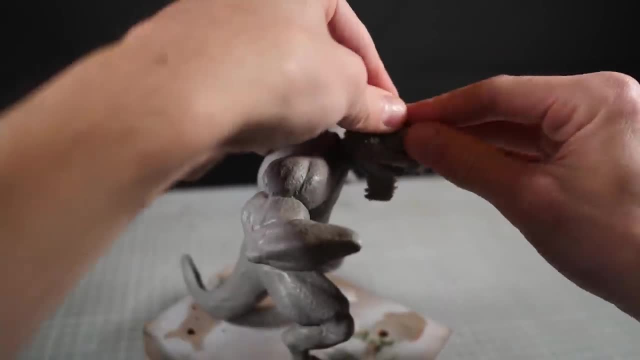 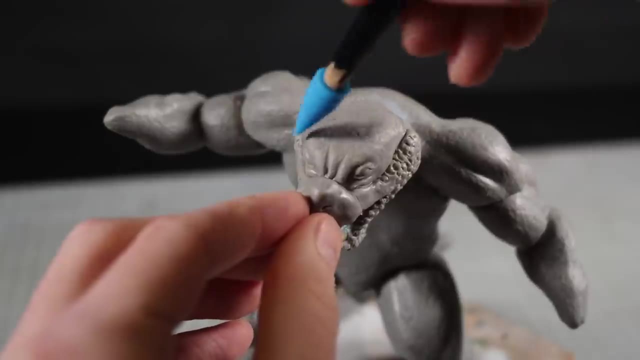 mostly finished. I can attach it to the body before adding the finishing touches. The neck gets blended into the body and then I can add a little bit of texture via my roller and clay shapers. Now is it just me, or does a bald, super jacked, hornless Bowser look a little like Kimbo Slice? 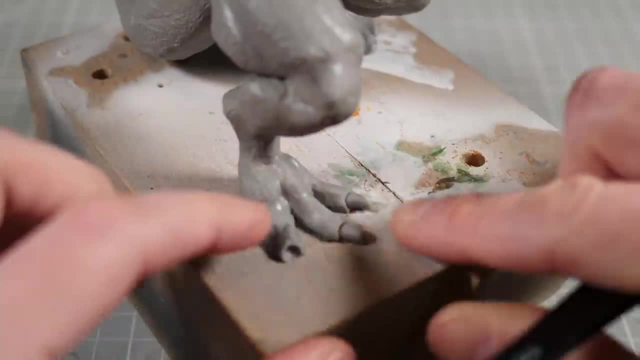 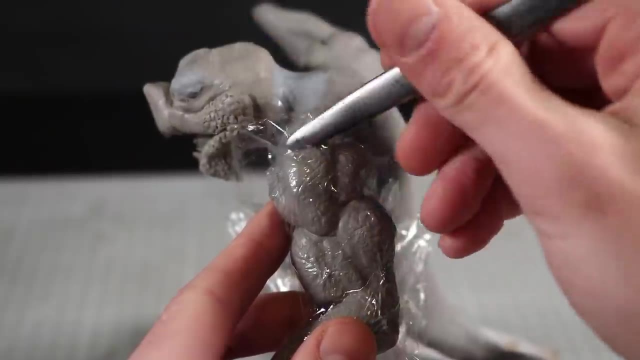 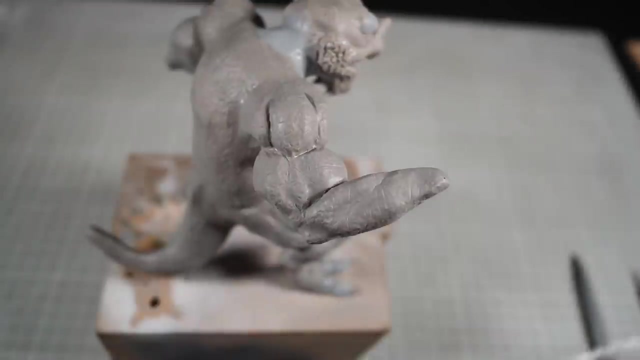 Anyways, I poke some dents into his toes so that I can add some talons to his claws. then, using the old cling film and shaper trick, I'll add some scars and skin marks. Finally, as some additional little highlights, I'll strategically smoosh some tiny balls. 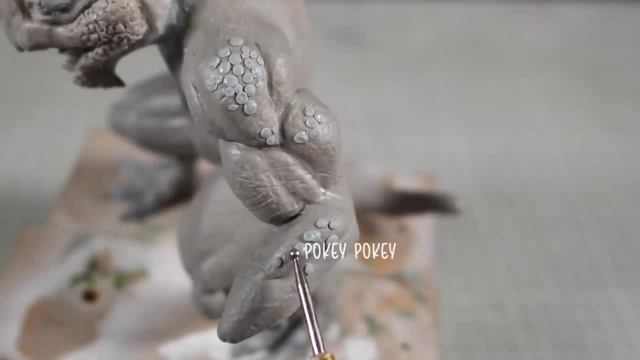 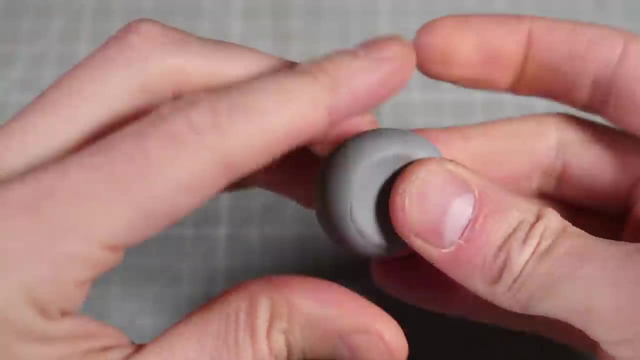 around his body and then blend them in by way of the old pokey pokey, And then a couple big pokes will give me a place to place my horns, and then I can get started on his hands. These start out as blobs of clay that will either get curled into an angry, ferocious 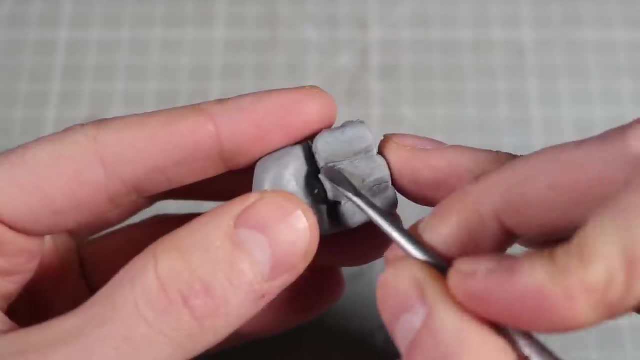 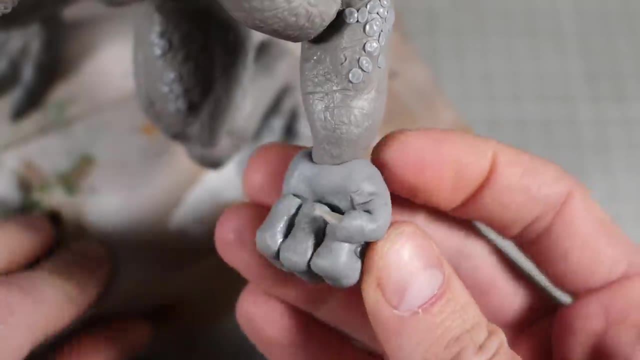 fist or an outstretched hand. With the fist, I find it's easiest to start with a mitt, then cut some fake fingers out, rather than making the fingers individually. Then I can simply add the thumb over top and stick it onto my arm stump. 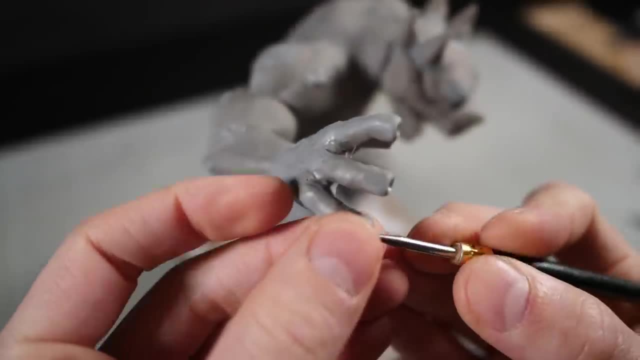 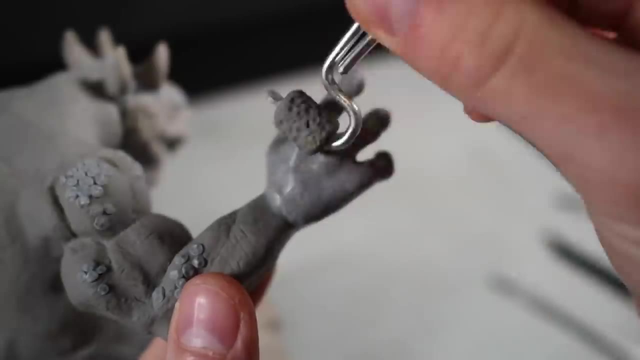 The outstretched hand, though, will have the fingernails exposed, so, like I did with the toes, I'll poke some dents to allow for little talons to get popped into place. then I can blend it in using a bit more texture, like I did with the rest of the arm. 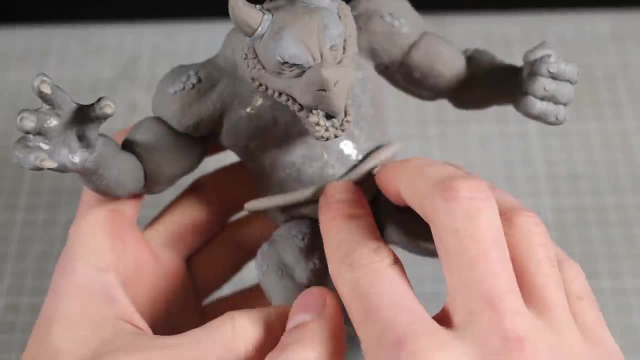 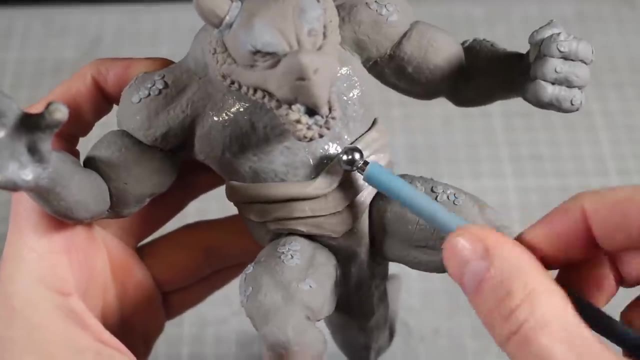 And it's time to get to work on his scaly Bowser belly. I'll start by rolling out a whole bunch of little wormy dealies, then pressing them into place using one of my oversized ball styluses to give it a bit of an interesting texture. 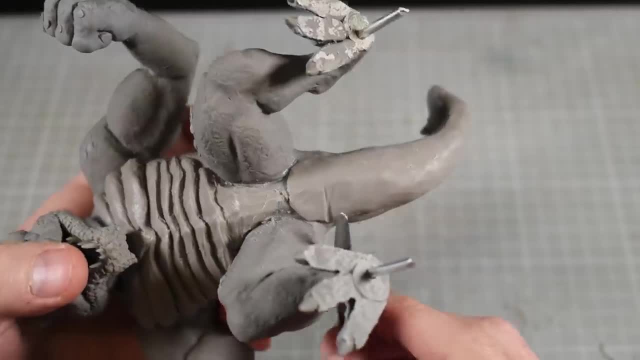 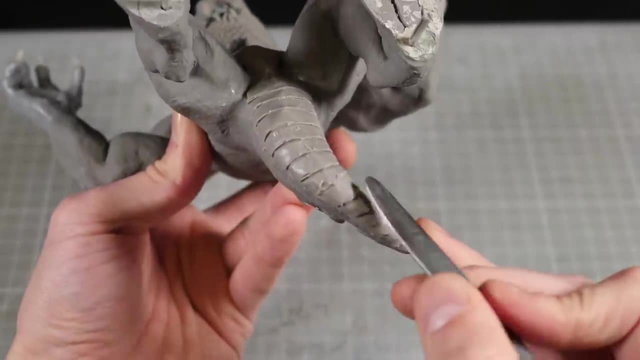 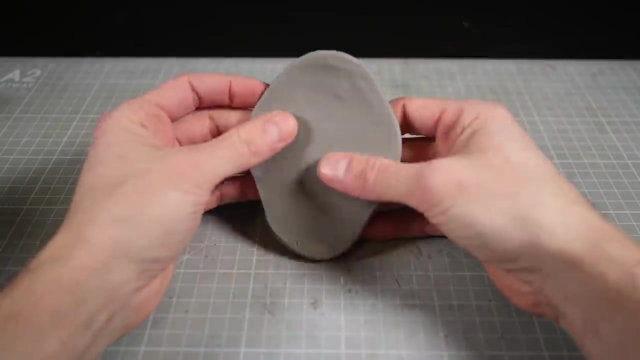 And I can add his scaly banana hammock and work my way down the tail, carving out the individual armour plates. Of course, what's a King Koopa without his shell? I'll start by smoothing out the tail. I'll start by smashing a ball into an appropriately shaped flat chunk and then get the right angle. 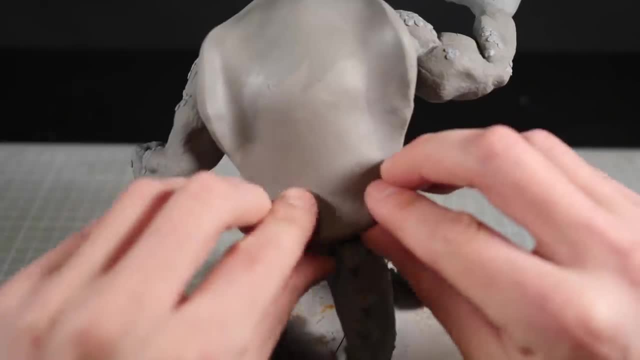 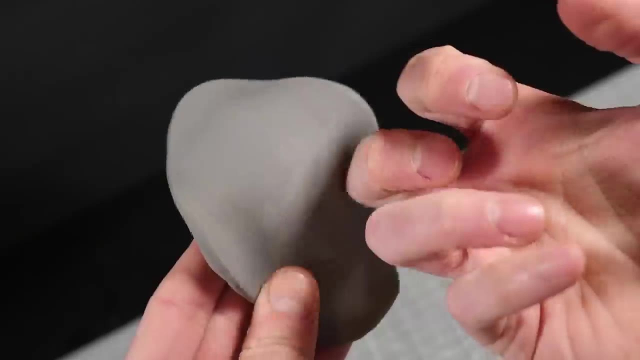 by shaping it onto my already baked Bowser body. Then I'll bake the entire thing in the oven to make sure it retains its shape so that I can use it as a base to add the detail. Because it's been baked, it's easy to use a knife and some files to create the segmented 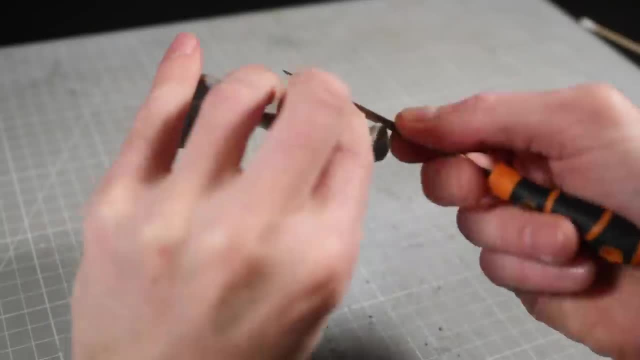 sections as well as create a lot of the nicks and scrapes. Then I'll paint a little bit of bacon bond over the entire surface so that I can add the top section over top. This will get smoothed out until it's just about done. 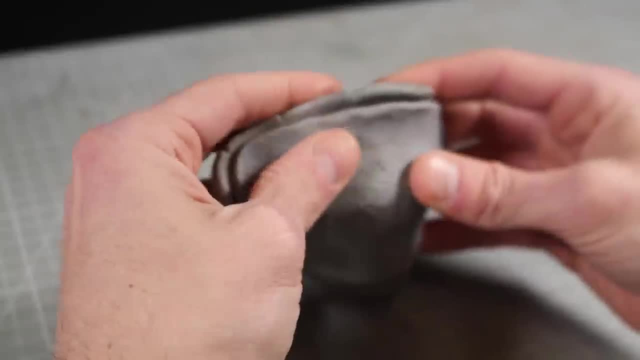 And then I'll add the rest of the parts, And then I'll paint a little bit of bacon bond over the entire surface so that I can add the top section over top, Just a few millimeters from the edge, and then I can add the individual sections of. 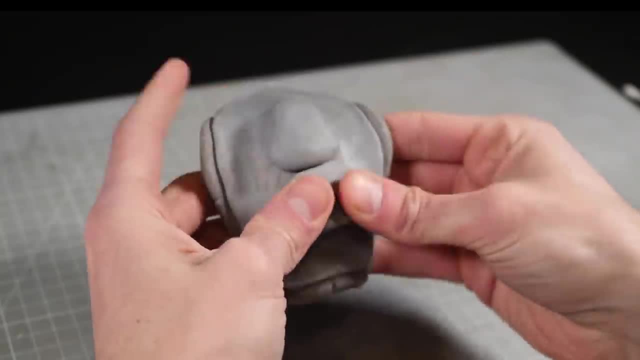 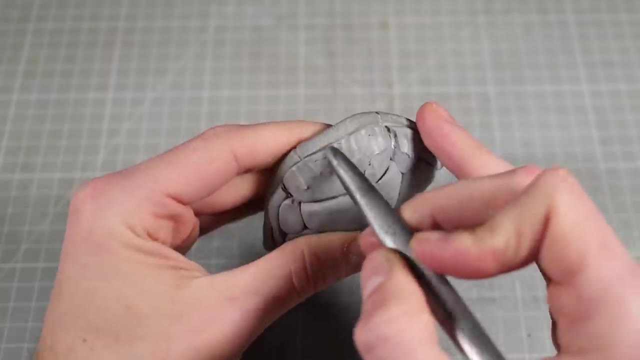 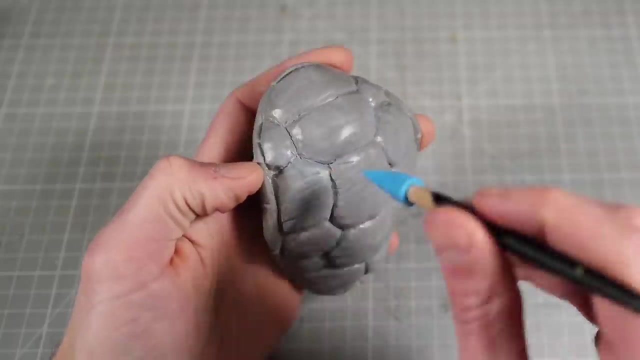 the shell. Once I've covered the shell, I can blend the edges and sharpen the divides between the sections before using my ball stylus to add a semi-smooth texture. Then I'll add some nicks and cuts before poking big indents into each of the individual. 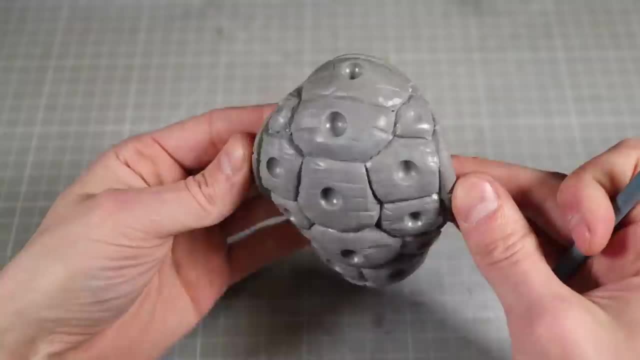 sections. These indents will be housed in the shell and then I'll add the rest of the parts. Once I've added the first section of the shell, I can add the final cleaning touches to them, calling them base, just to add a little bit of fun to the shell as well as adding 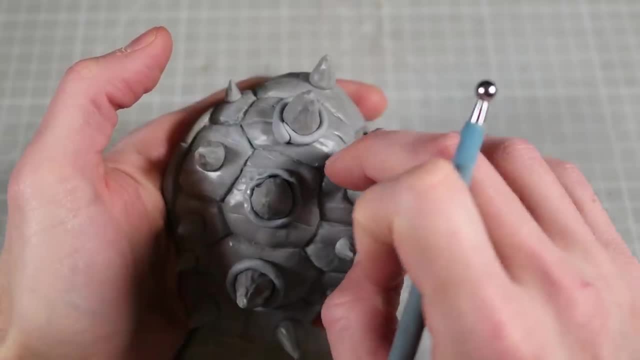 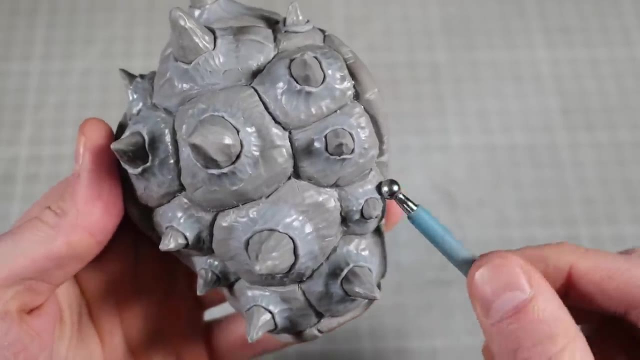 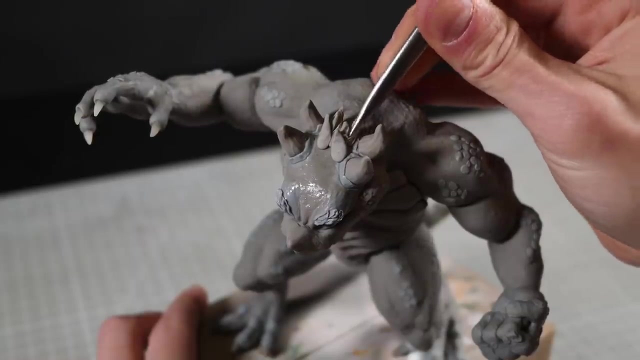 a little detail to the base, And then I'll add a little bit of the other details, like the base of the shell and the base of the shell. Finally, I can add the final details to Bowser. These will include his eyebrows, the little patch of hair on top and his various emo. 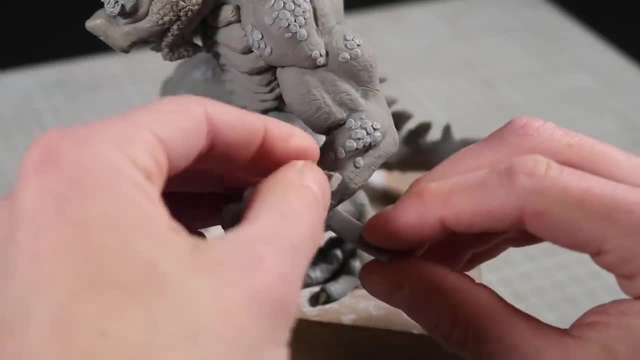 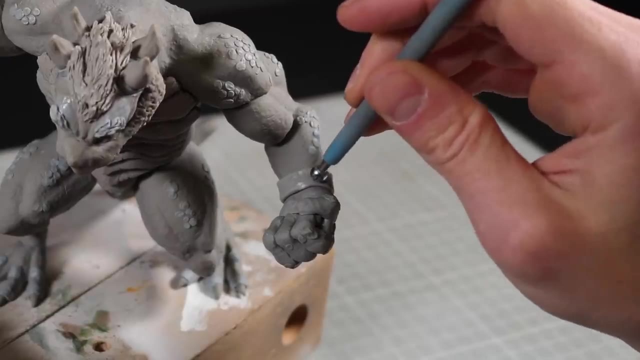 bracelets. Now, before I catch Hal in the comments, I know that I've left his biceps bracelets out, but I couldn't find a way to find out if he's doing any work on his shoulders to fit them over top of his ridiculously large muscles without them looking silly. so I'm 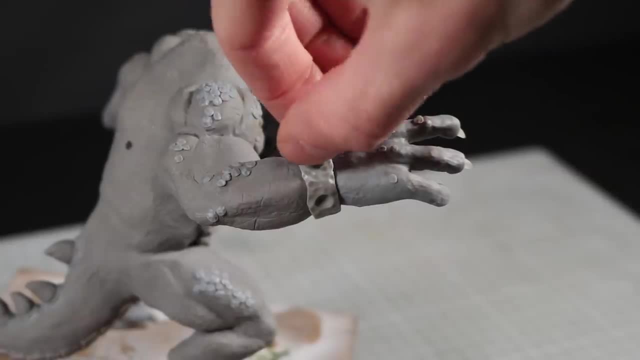 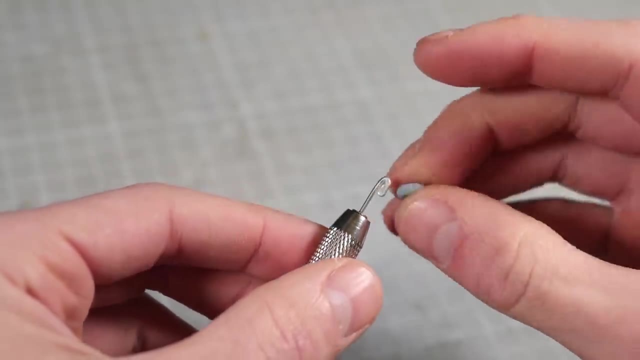 just going to go with artistic license and not do them. Otherwise he's finished and ready for one final bake, which means it's time to get started on our tiny Italian plumber. I wanted to stick with a semi-realistic style here, but I also wanted Mario to retain his. 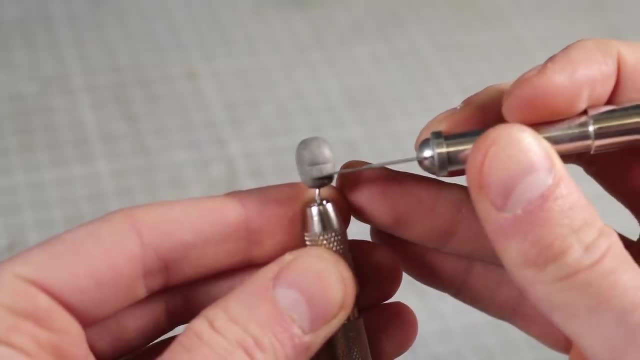 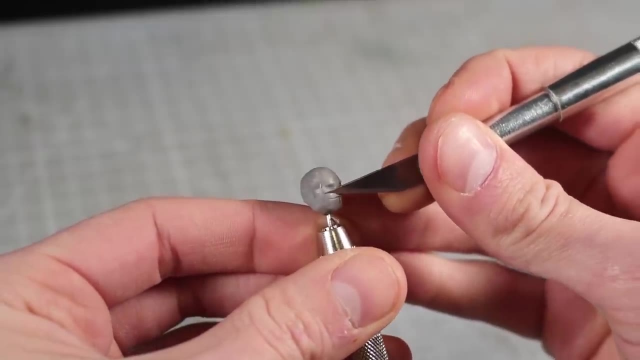 characteristically ill-proportioned body, so I'll start by making his head, so that I can get the rest of his body to match the correct size- or incorrect size, I suppose, is more accurate. Making his head follows the usual guidelines, though, so I'll mark out the center line. 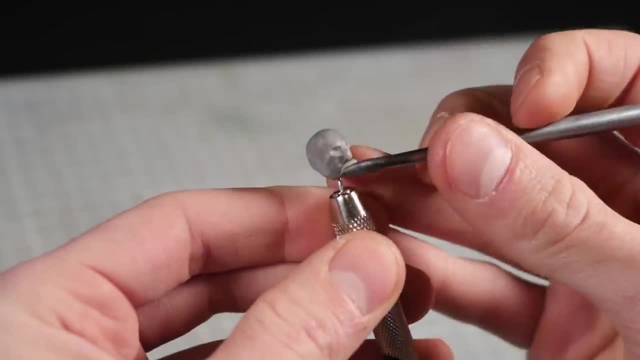 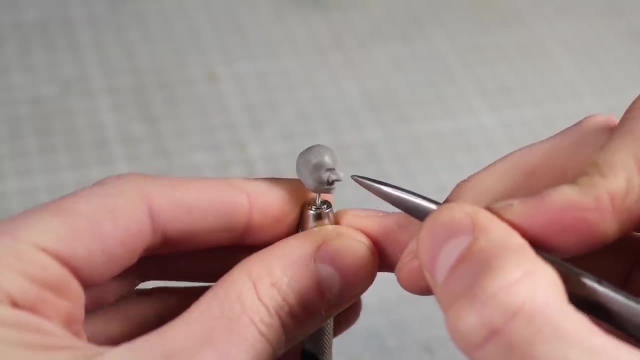 as well as the eyes, nose and mouth. then cut the cheeks down to give me my shape. Then I'll add his oversized nose and strong Italian chin. I also only need to make his bottom lip, since I'll be adding his trademark plus size flavor. 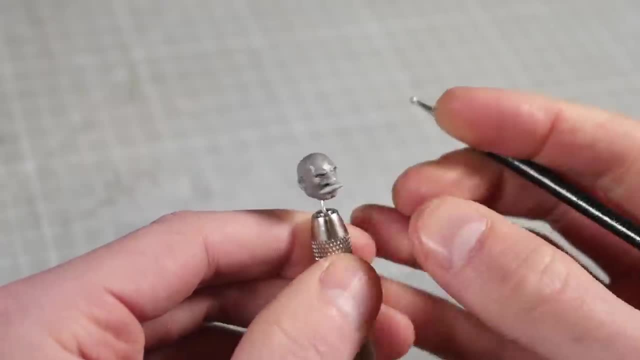 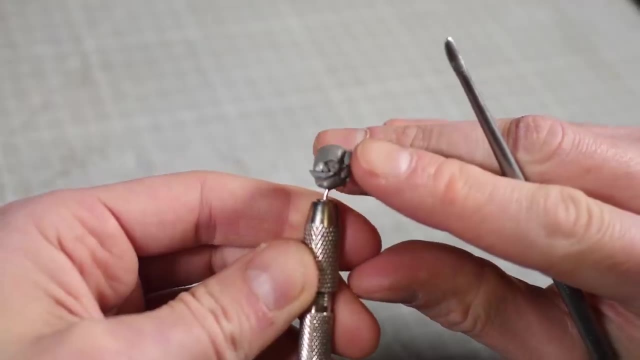 saver later. Now I was trying to figure out before I got started what kind of style I wanted to go with for Mario. I considered the poncho. I wanted a ponchy kinda chubby, somewhat comedic look, but decided that if Bowser is, 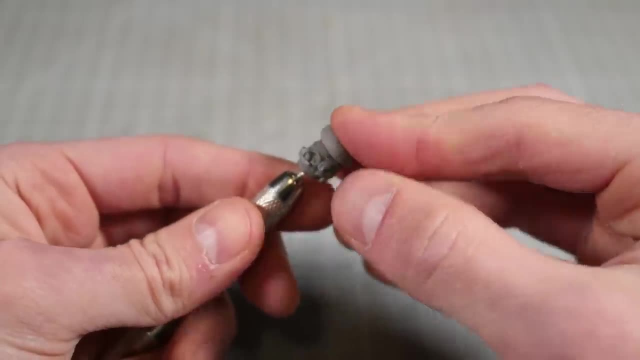 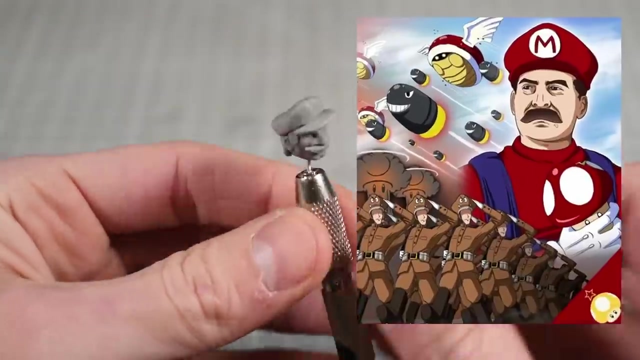 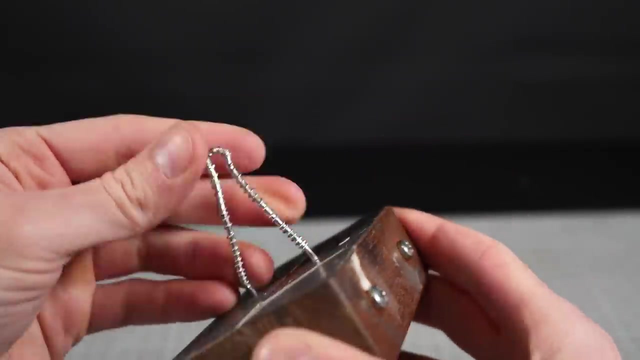 gonna be a big, 15 foot tall bodybuilding monster, then Mario needs to be appropriately heroic. So naturally I settled on the square-jawed superhero you might see on a Soviet Union propaganda poster. Of course, if I've gone with the square-jawed Joseph Mario, then I need to make sure his 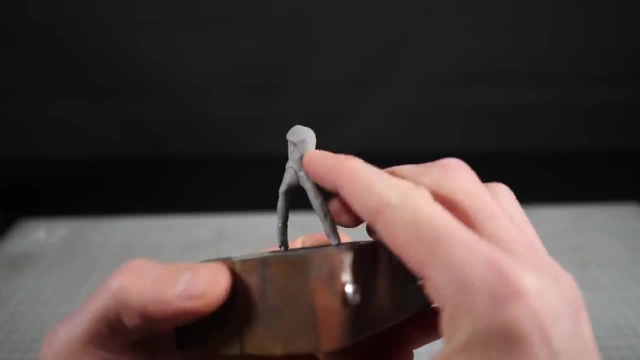 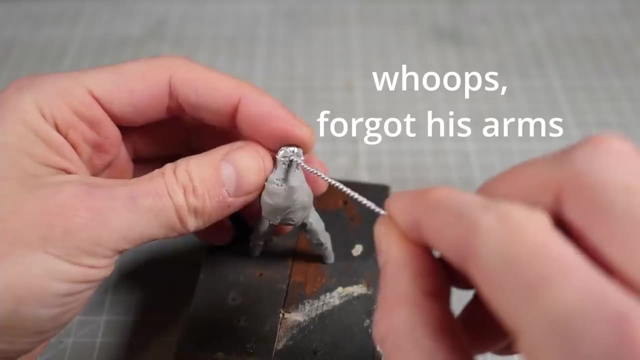 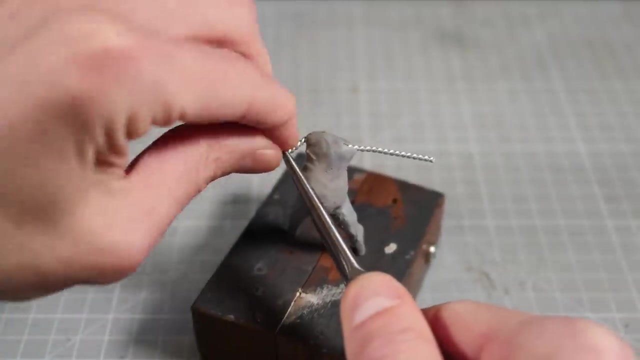 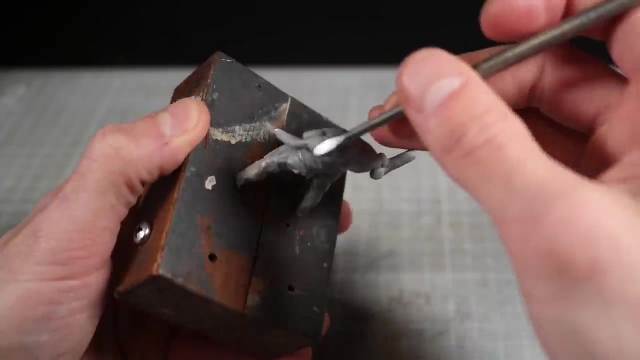 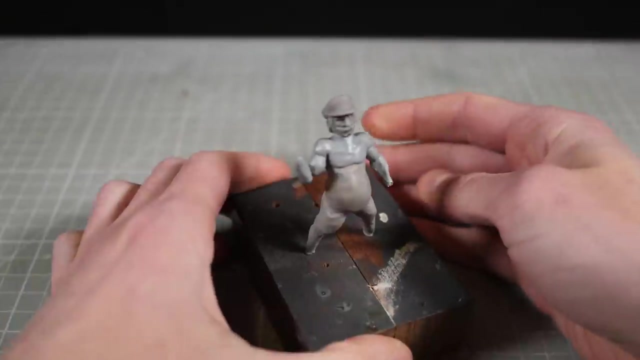 body fits the theme as well. so I decided to go with that beer-bellied lumberjack look. You know the look: The big round gut, but tree trunks for arms. Now just try and tell me that's not the ideal Mario body. 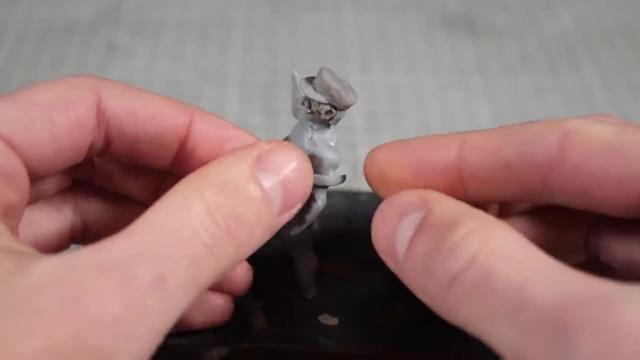 So all I need to do, then, is add the clothing on top, and the easiest way to do this is just to add little bits of clay around the body. I'm going to add a little bit of clay around the edges and then blend them in so that. 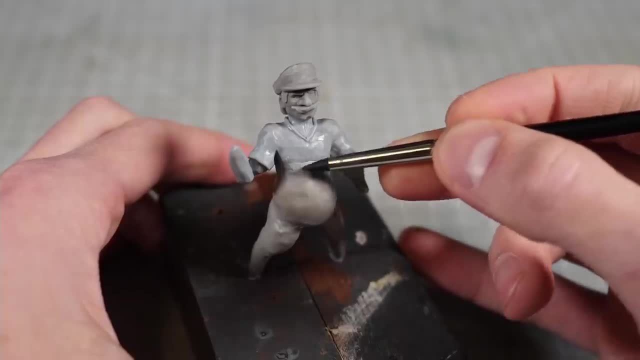 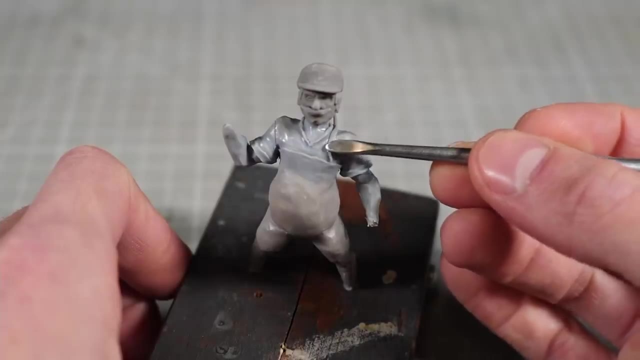 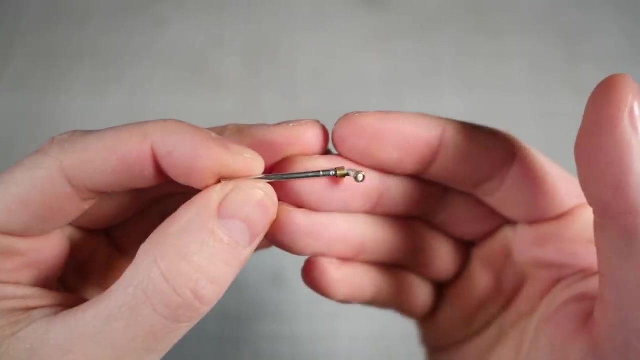 he looks like he's almost too buff for his shirt And I can fill in any of the gaps and add his overalls. His boots are just basic little leather lumps and I made him a mighty pipe weapon out of armature wire and brass tubing. 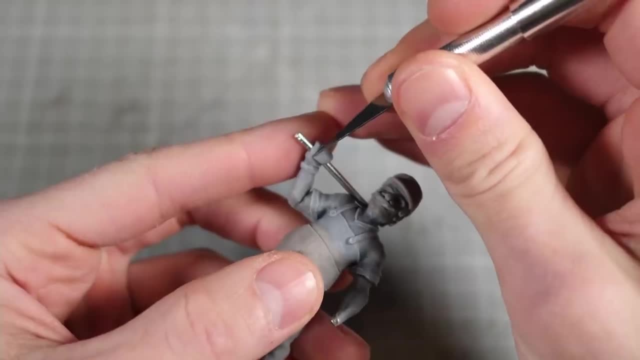 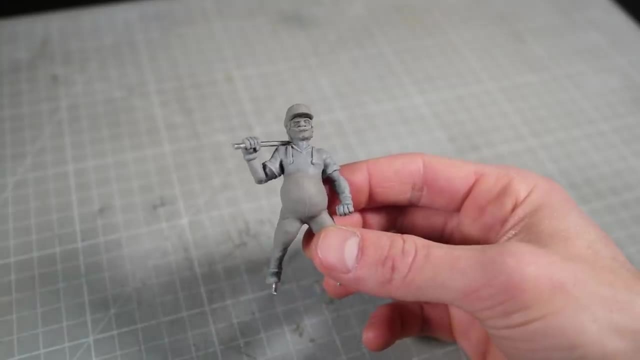 He'll be holding this defiantly over his right shoulder as he strikes what might be the single most heroic pose I've ever sculpted: Waha. Finally, however, we're onto the painting, so I'll start by flicking him until he's primed. 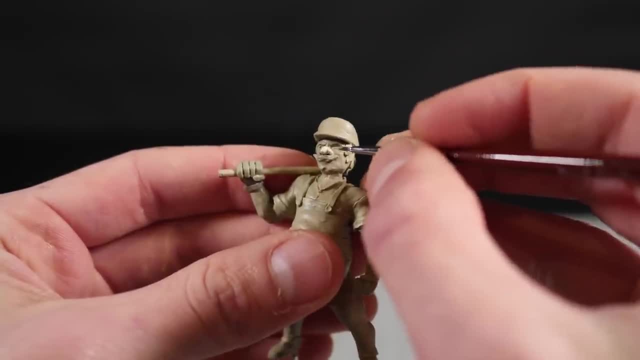 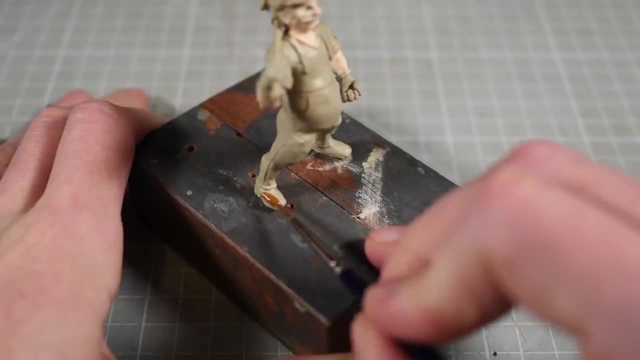 in beige, And I'll start by laying down my base coats and working my way up to the smaller detail. I've decided to stick with Mario's basic red and blue theme because I like it and it's quick and easy, which makes me like it even more. 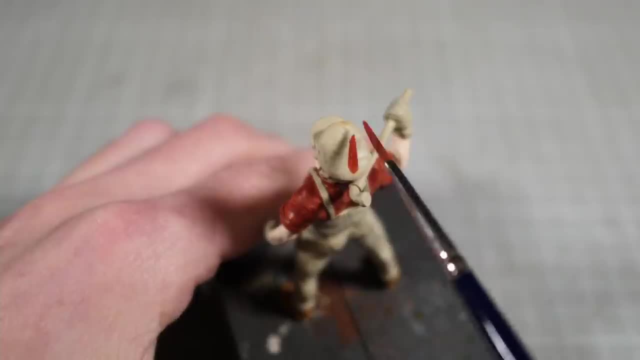 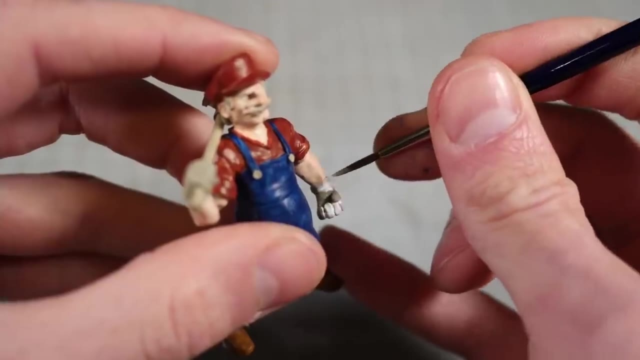 I'll paint his leather boots with a leather brown, then his shirt and hat get a nice red coat and his blue jean overalls get a coat of blue jean overall blue. Then I can paint his little white gloves white and get to work on those details. 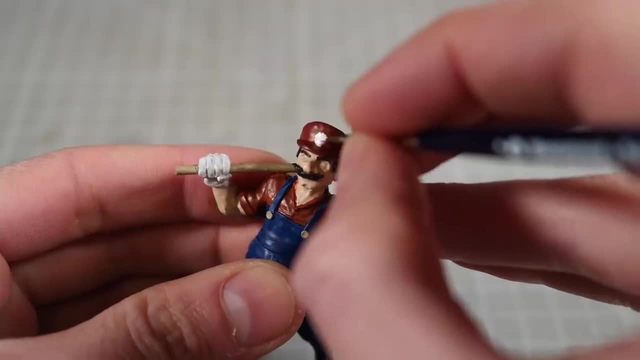 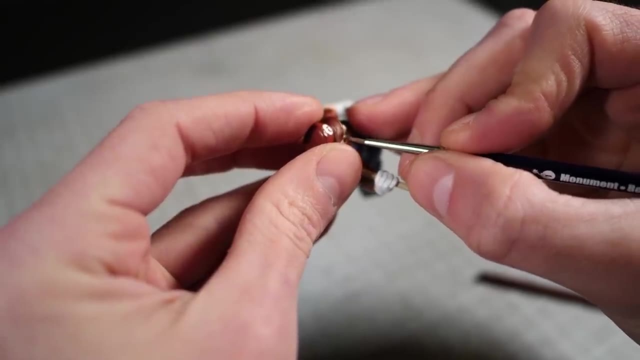 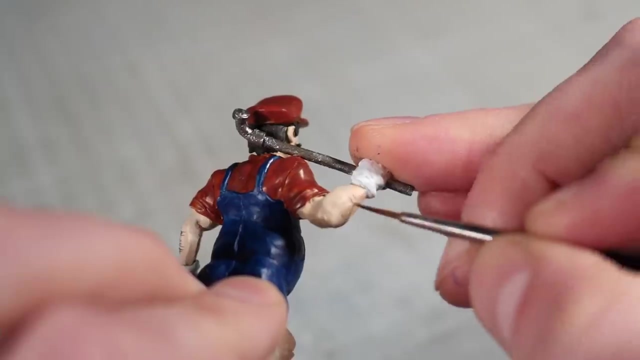 Tiny little details. Pro tip here: if you've got the shaky hands of a middle aged alcoholic and you're terrible at painting eyeballs, then make sure to angle the camera in such a way that no one can actually see what you're painting. Finally, with this, plus two pipe of Koopa slang painted gunmetal grey, I'll add some manly. 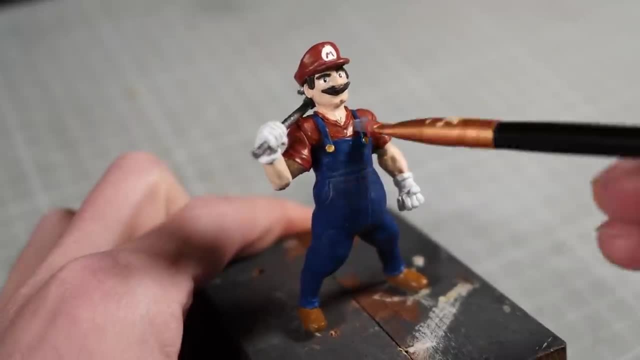 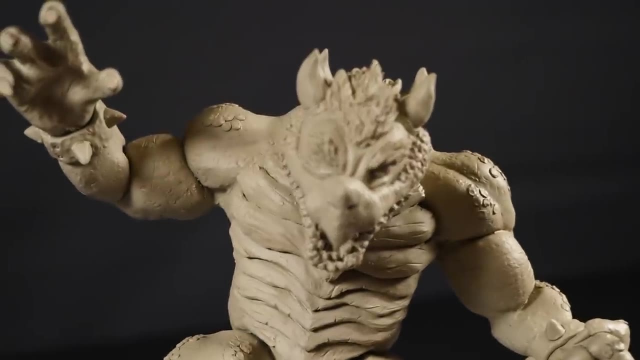 arm hair, before giving everything a quick dry brush with lighter tones to highlight some of the edges. then it's on to painting the mighty king of Koopas himself. Same as Mario, I started with a beige primer. This is particularly important since I want to paint Bowser- mostly orange, and orange is. 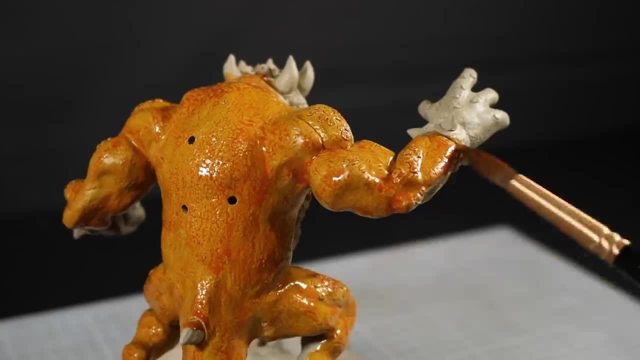 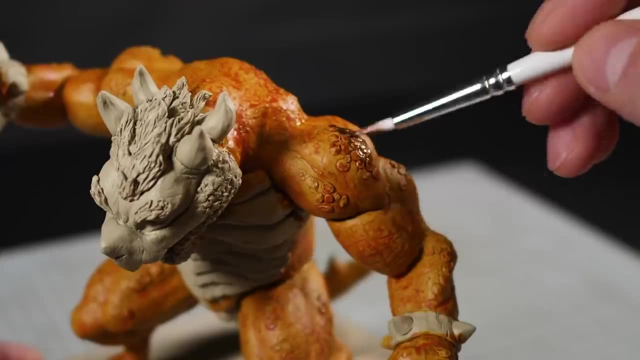 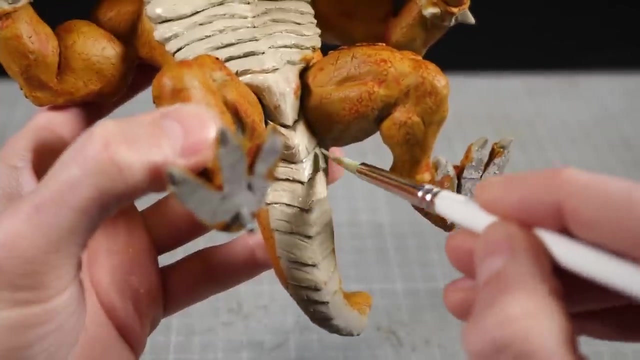 notoriously hard to get a good coat. I am, however, using contrast paints which are pretty heavily pigmented but should settle into all the surface textures quite nicely. I'll give the raised areas a quick wash with a darker colour to make them stand out, before painting his chest and bony extrusions with a bone white. 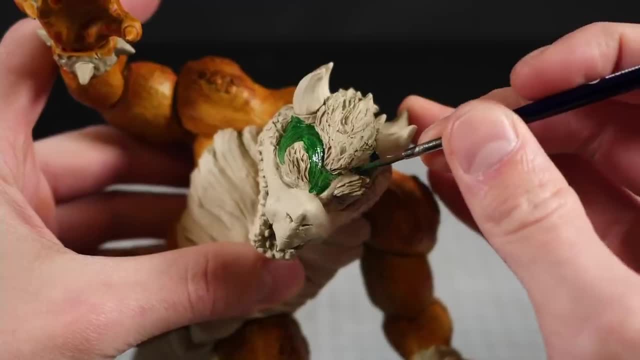 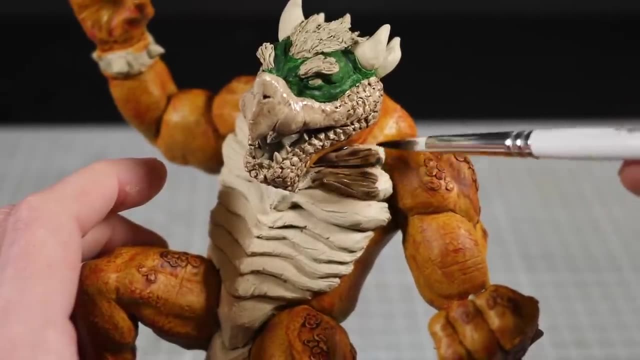 His trademark green head will get painted… well, green. and then I'll go over all the bone white sections with a sepia wash. This gets into all the cracks and adds easy shading, but also helps to give all the horns, bones and armoured plates a nice weathered look. 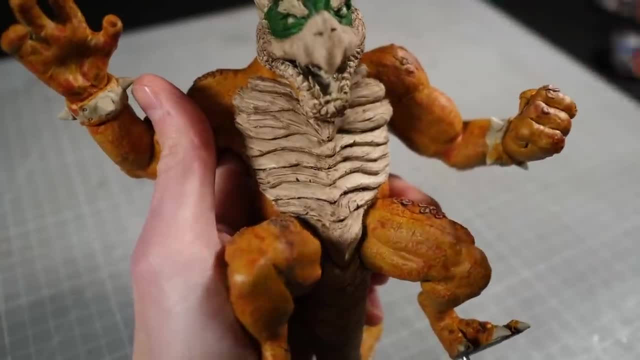 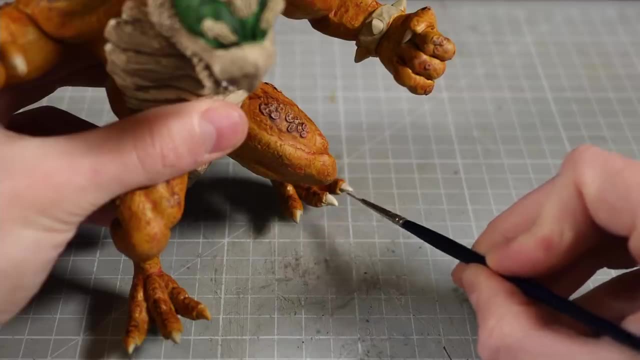 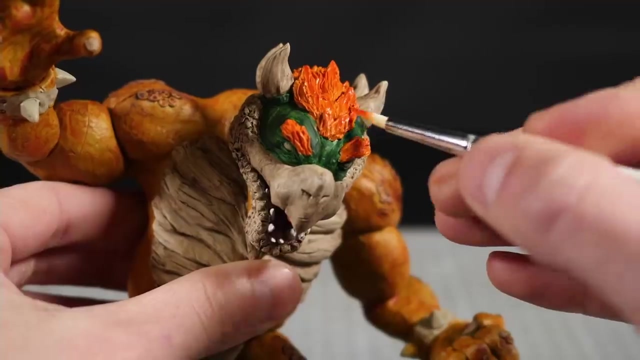 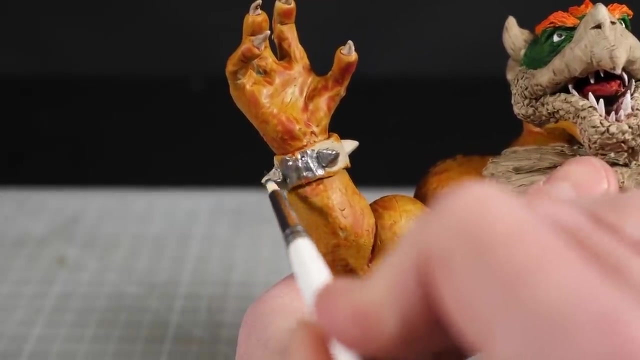 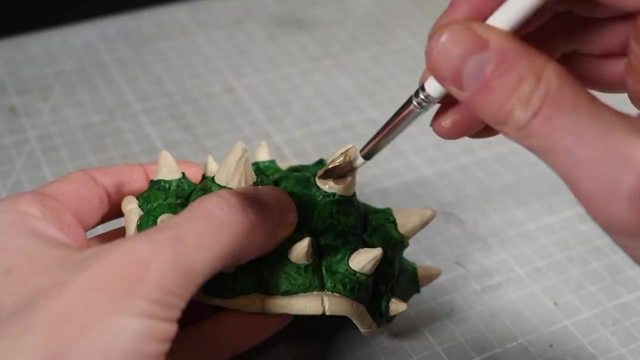 Finally, everything gets a quick dry brush to help sharpen the edges, and then I can get started painting in all the finer details. Now I considered giving him a blue shell, but thought that was just crazy. so I got the traditional green base coat, followed by bone white spikes and a sepia wash for colouring. 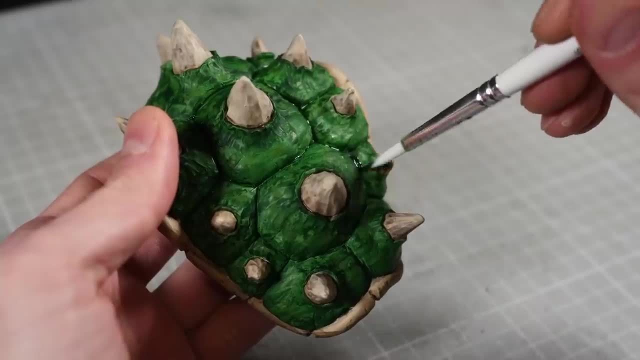 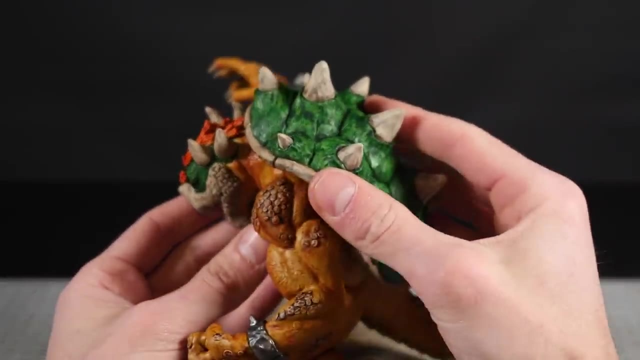 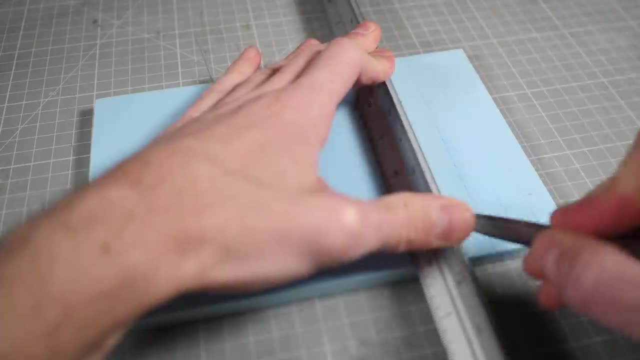 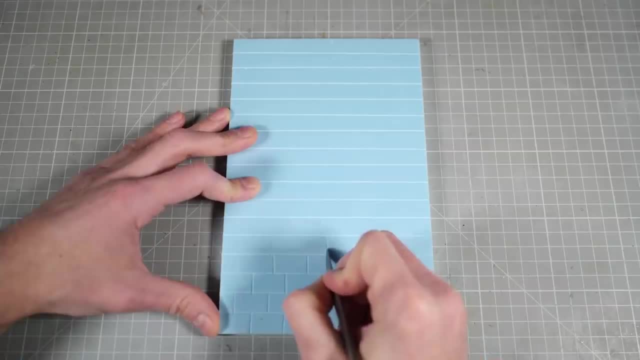 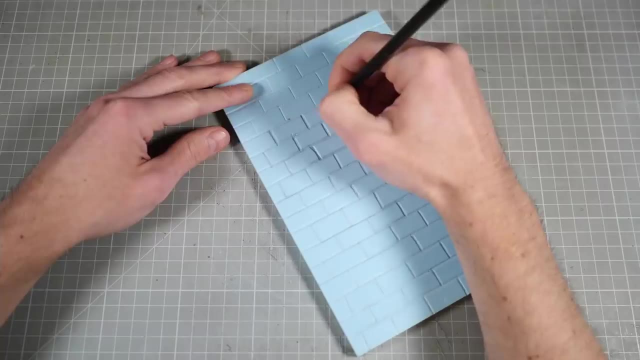 flooring. Then I'm going to add the vertical cuts to separate the lines into individual bricks, and using a dull pencil I'll retrace the lines, which will give the bricks a lot more depth. I'll also cut some of the edge bricks off so that it's a bit more interesting. but 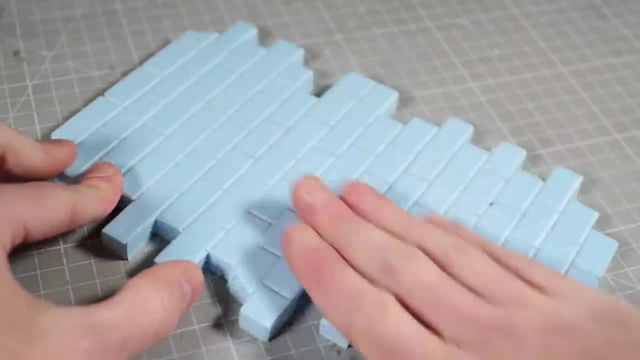 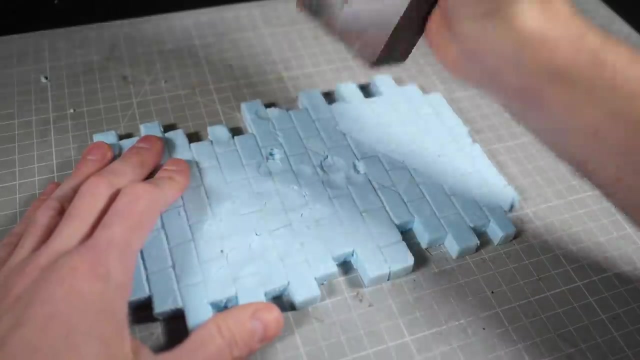 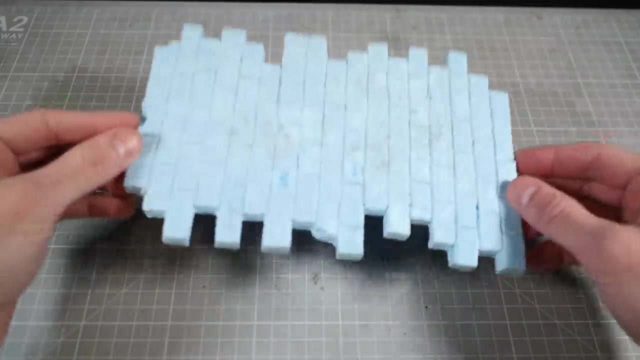 apparently I didn't film that part because I'm bad at my job. Otherwise, I'll use a couple different materials to carefully add some surface detail and, with the detail done, I'll give it a quick coat of black Mod Podge followed by a gray base. 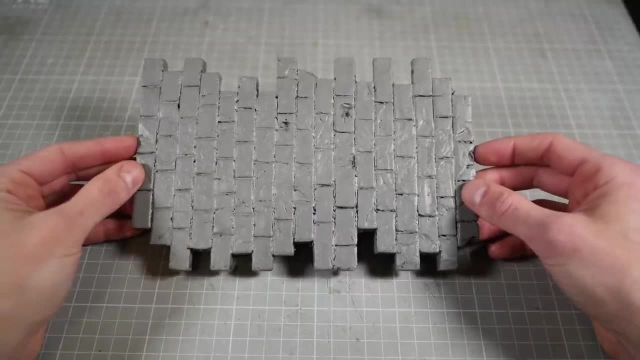 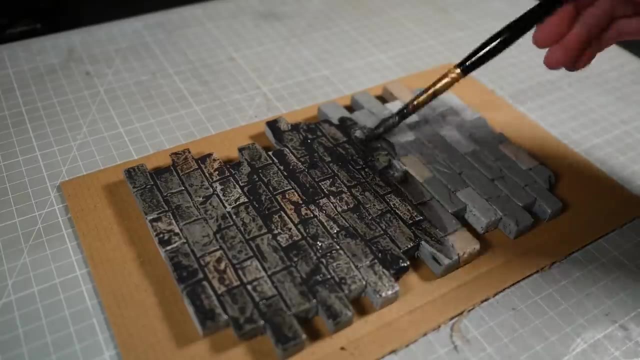 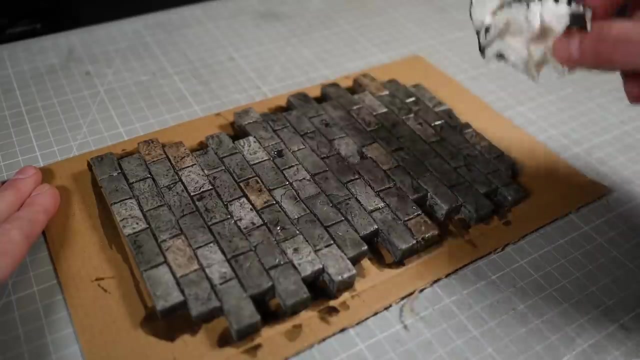 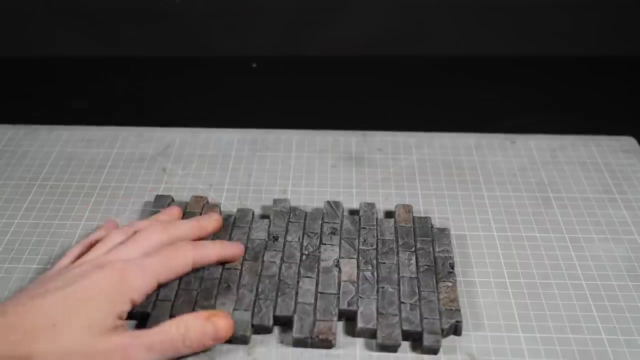 coat and I'll paint a few bricks with different shades for variation. then the entire thing gets a heavy coating of black wash and then finally, to make all the edges and cracks really stand out, I'll give it a dry brush of light gray, followed by white, and all that's left to do. 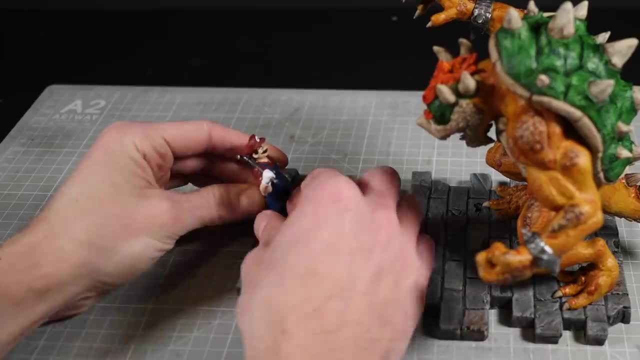 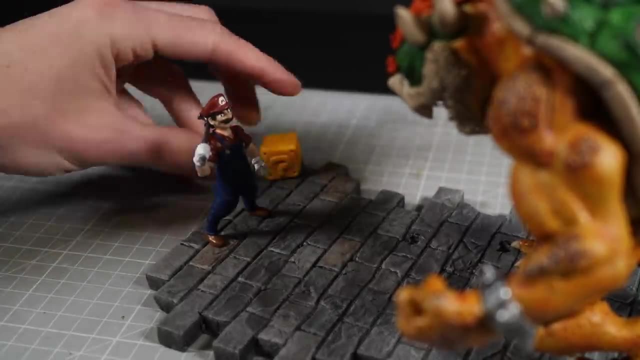 then is stick our dynamic duo in place. however, once I'd gotten Mario in place, I realized it was a little empty and I didn't want to overload the base too much. so I made a tiny question block and a whole slew of hallucinogenic mushrooms, and then I painted the base with a black paint. 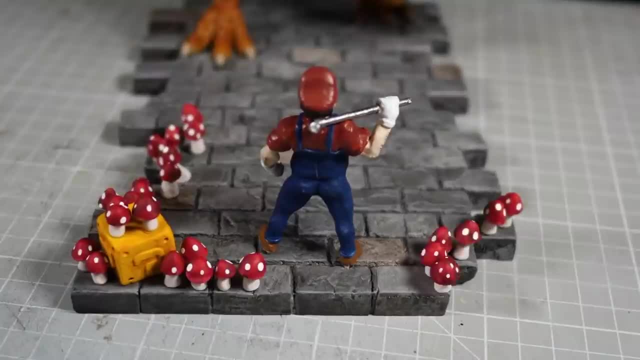 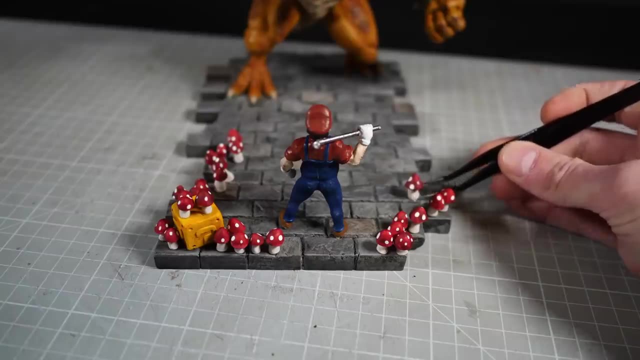 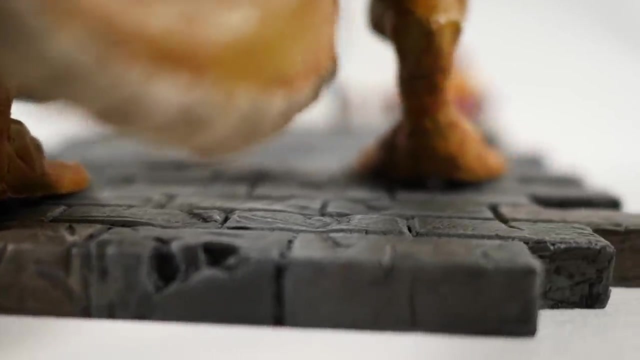 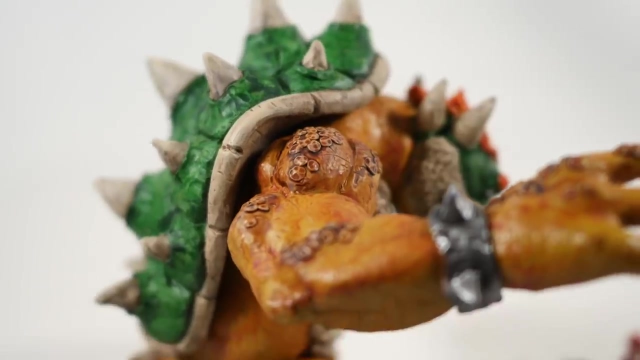 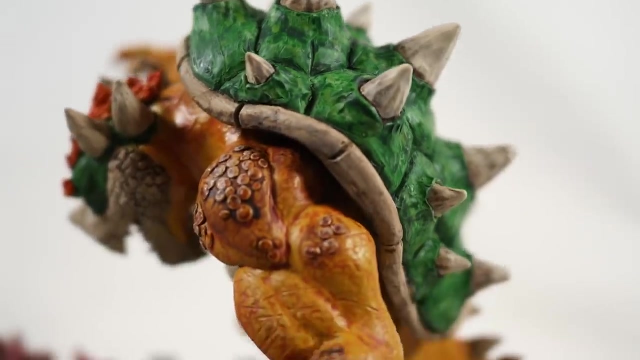 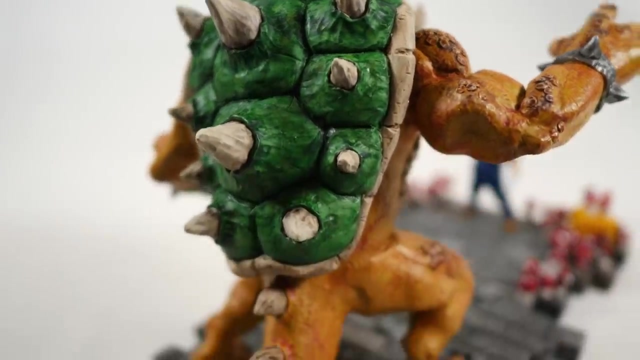 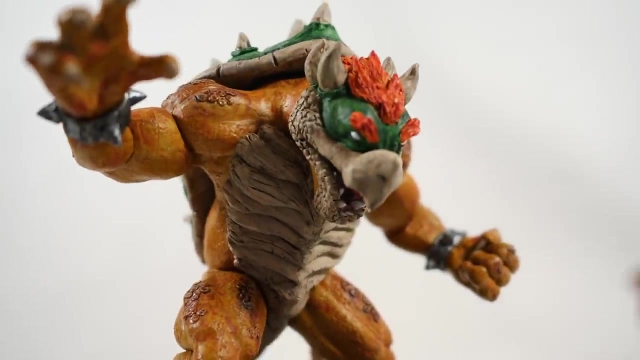 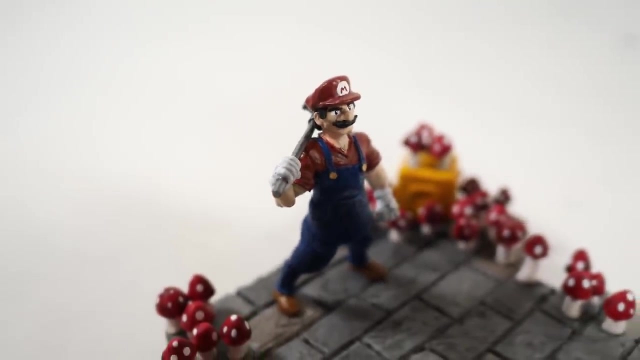 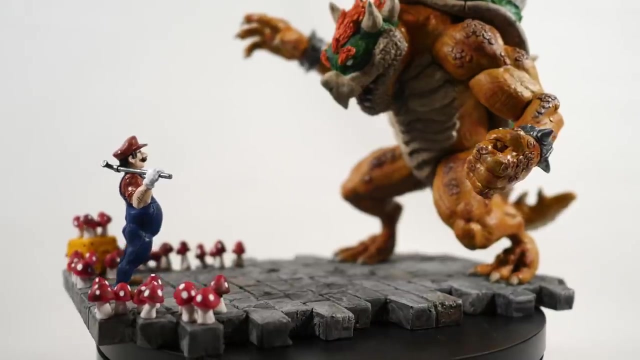 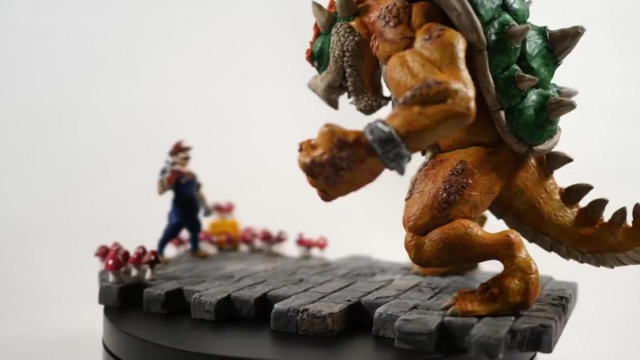 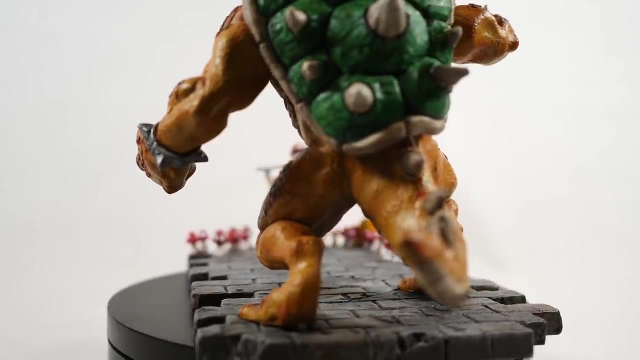 to help build up Mario's side. so, with our mushrooms in place, we're on to the glamour shots. then I just spited out the theme, and so you can download it, and download it right in there. as always, a huge thank you to the folks over on patreon who help make these tiny nerdy things a.